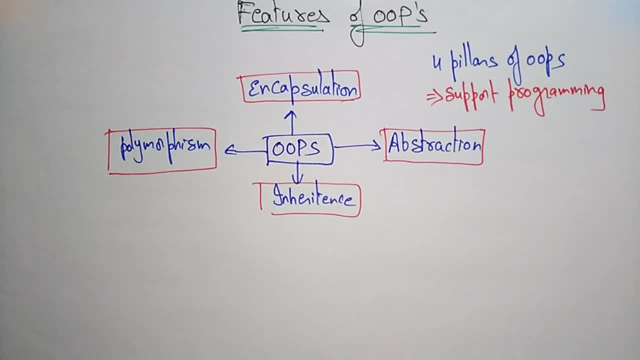 one is the abstraction. so what you call this abstraction, so abstraction. so abstraction is nothing, but it is a abstracting. the data suppose? uh, it is, it is nothing but something only existing as an idea, only abstract is present. just suppose, if you take the example, as we say, abstract, 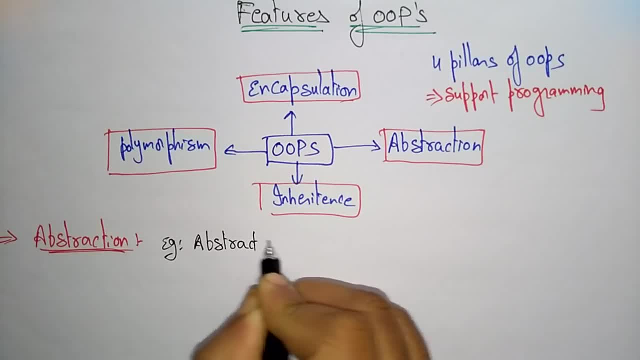 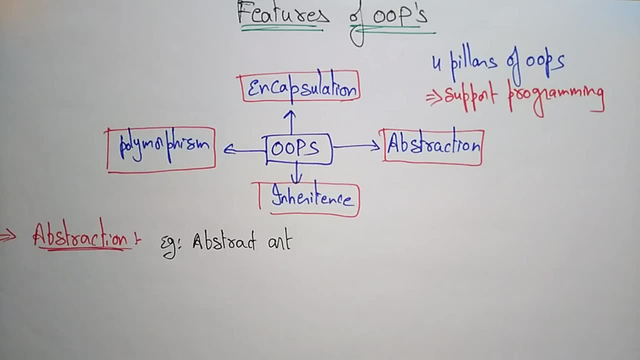 abstract art. so if you see the abstract act, you will just see a painting with a no image. okay, you call that is an abstract. ad means only that different colors will be spread on the sheet. then it will looks beautiful. okay, it doesn't consisting of any particular shape. 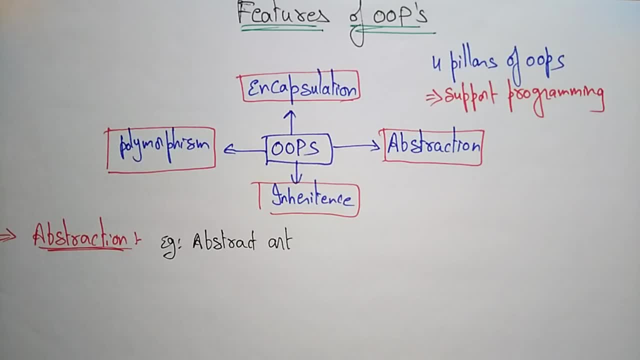 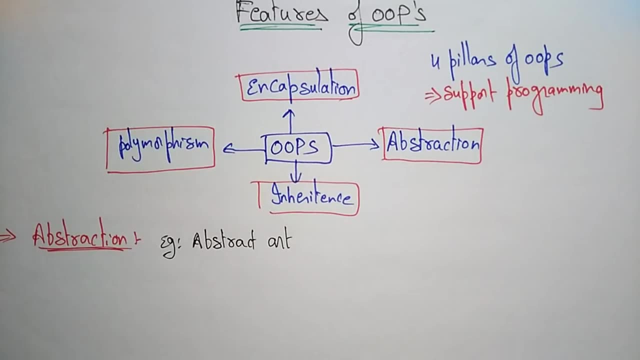 or nothing like that. okay that you call it as abstract art, it's. it only hides the implementation details. okay, so we call it a abstraction is nothing, but it hides the. it hides implementation details, implementation details, while just presenting- but evenatiellen just presenting- the features to the outside world, so it is just showing. 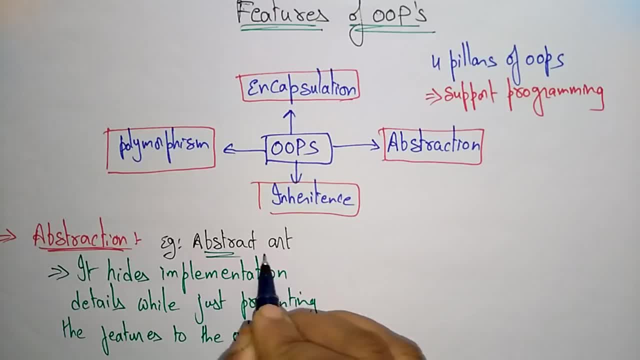 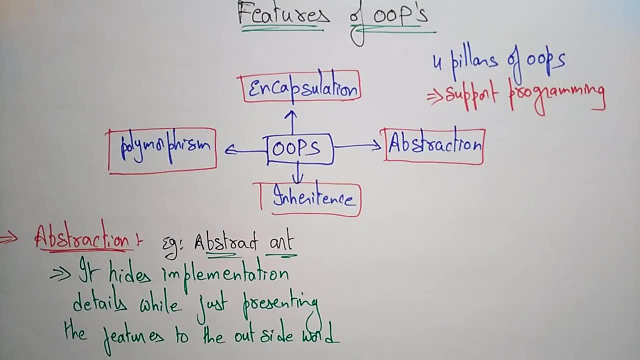 the features to the outside world. so if you see the abstract art, you just feel it. that the pink, the painting is beautiful, means only to the outside world. it just showing the features, but it hiding the implementation details, which means what colors, what colors they are mixing. okay, if we get one color, how many colors? 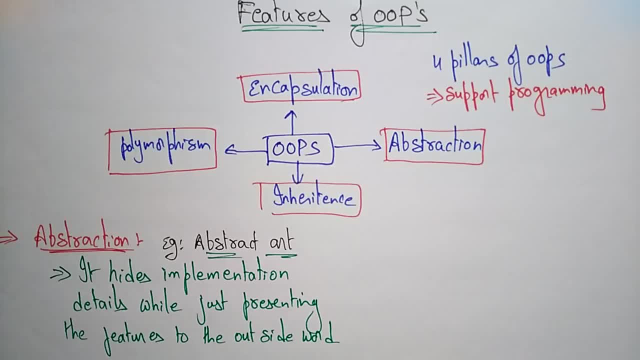 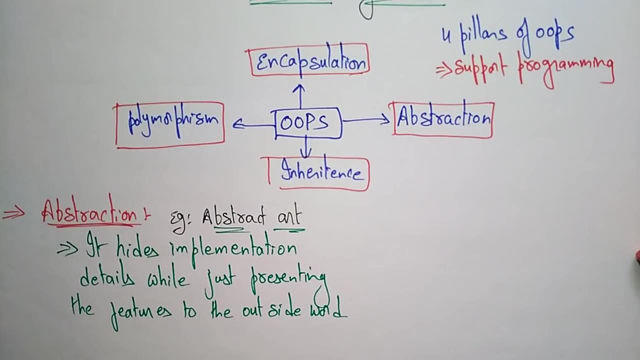 they're mixed up. okay, like that abstracting, it's hides the implementation details and it only focus exposed to the uh or outside world. only the features will be exposed to the outside world. okay, so coming to the main advantages of using this abstraction, so why we are using. 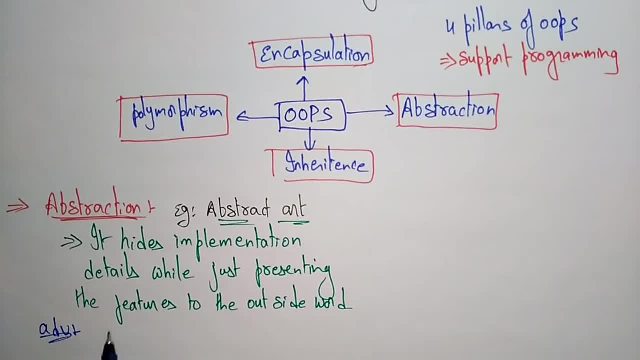 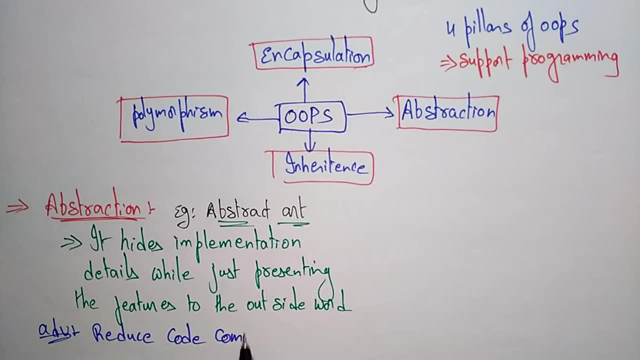 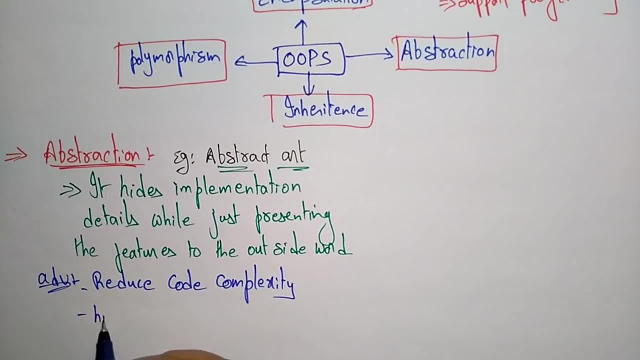 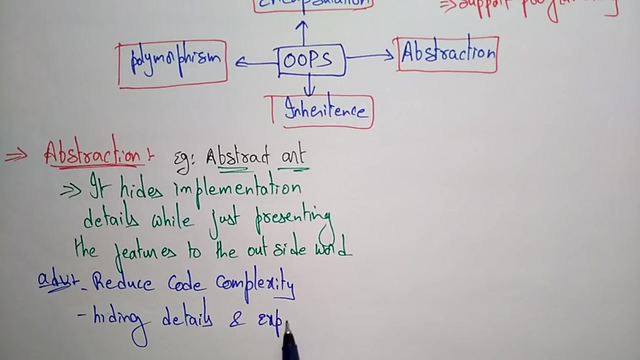 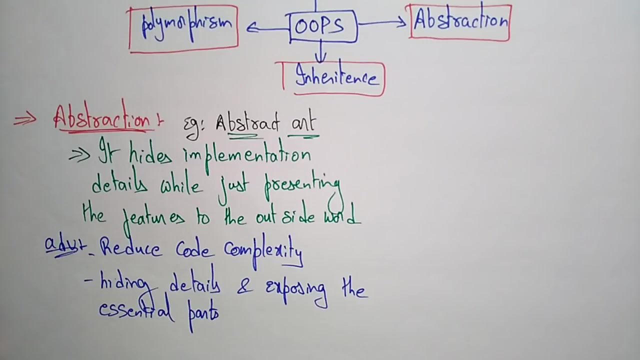 this abstraction the main advantages, or it reduced the, reduce code complexity, reduce code complexity and it hides the details, hiding details and exposing. so what it? exposing only only the essential parts, exposing the essential parts. okay, so abstraction: hide the details and expose only the essential parts. so i'll take one example to explain what is this an abstraction. okay, so if you take an example, 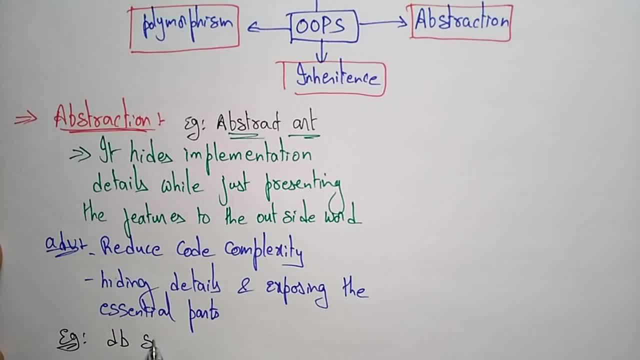 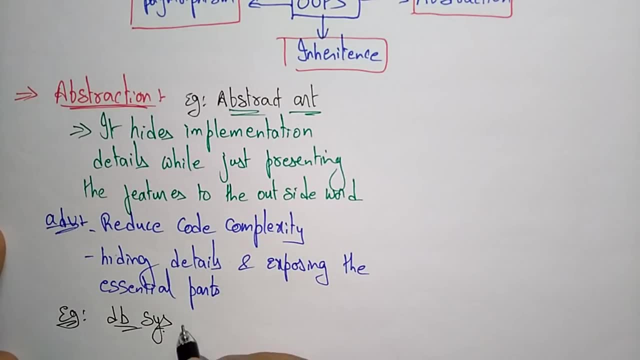 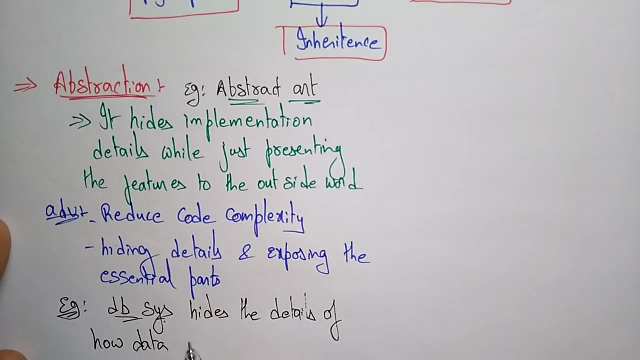 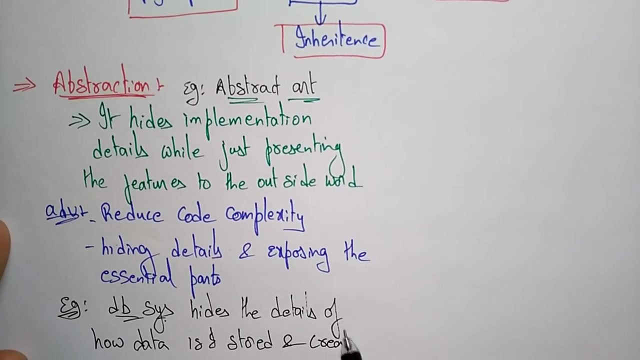 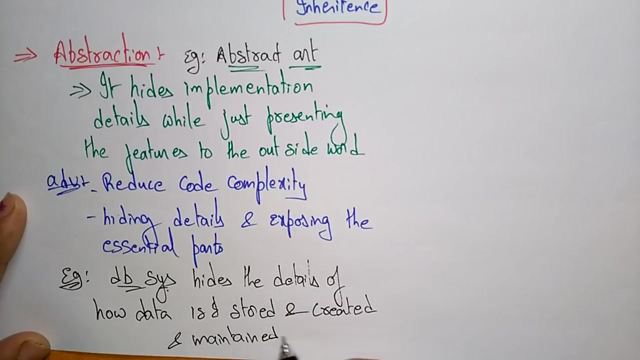 uh, database system. okay, so what is it? in database system, the abstraction will play a role, like it hides the details of, hides the details of how data is stored and created and maintained. did you get it? so? here the abstraction is saying in the, if you take the database system, the 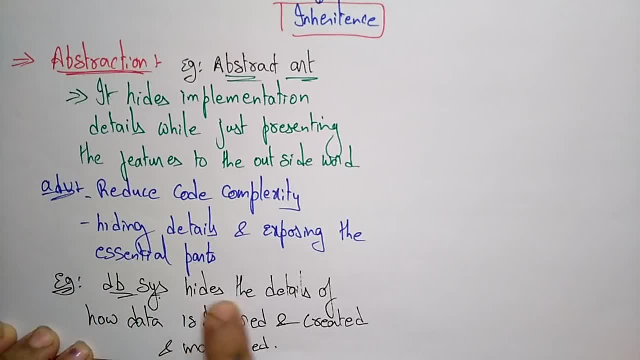 abstraction will play the role, like it hides the details of how data is stored. we don't know how the data is stored in the database, we don't know how it is created and we don't know how it is maintained. what we knows we only- uh, whenever we are just typing for information to see on the screen. just, we are. 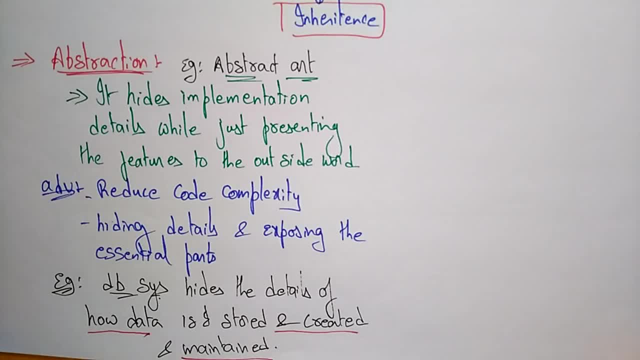 rising one query and you'll get the result on the screen, but the user doesn't know what it happens inside, how the data is stored and how it is created and how it is maintained means it is hiding all the details related to that particular table. it only the things which are essential to the person. 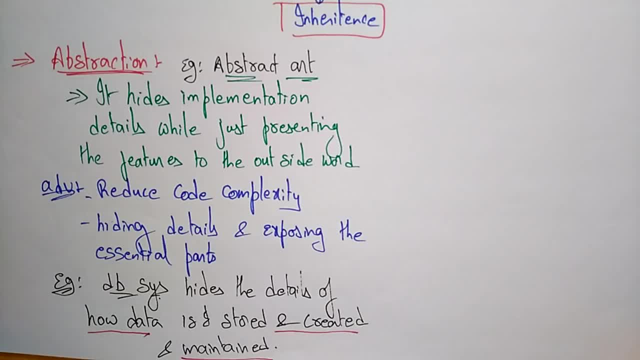 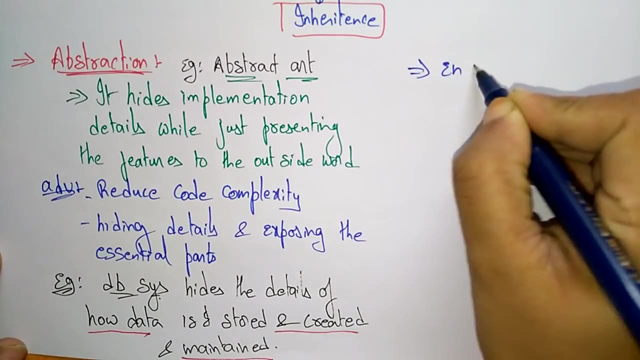 that only uh, exposed to the uh, outside world. okay, means it's hiding the details and exposing only the essential parts, that you call it as abstraction. so now let us come to the another thing, that is, the encapsulation. actually, the encapsulation and abstraction, both are. 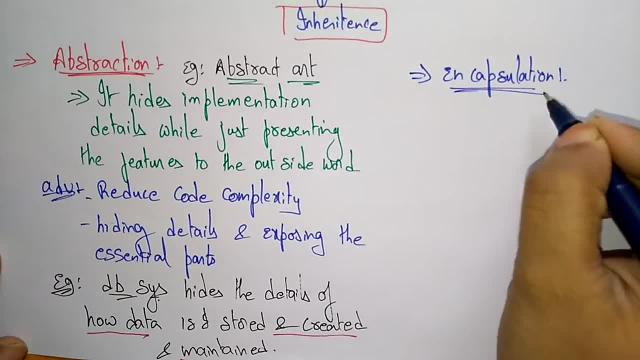 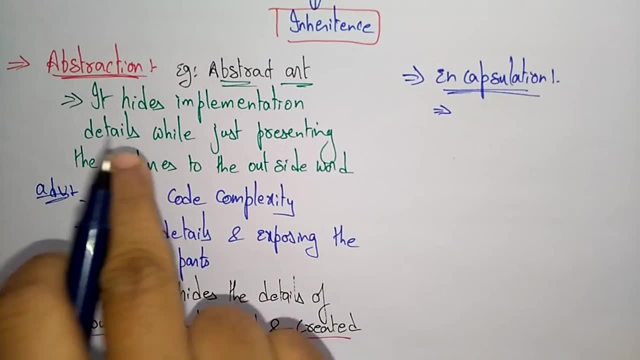 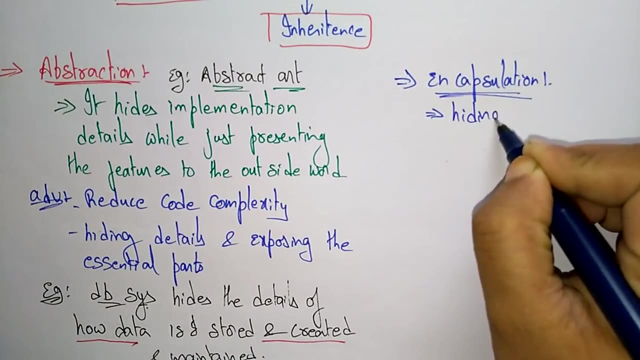 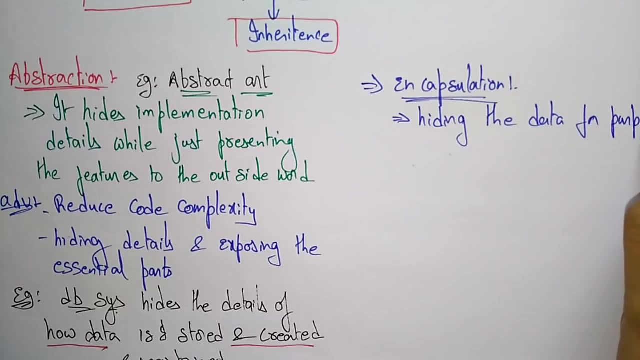 uh, almost almost equal say, but only the difference between: here is encapsulation hiding the data. it also hides the data, whereas abstraction is also hides the data and encapsulation is also hiding the data. hiding the data for purpose of purpose of protection. it's also hides the data for the. 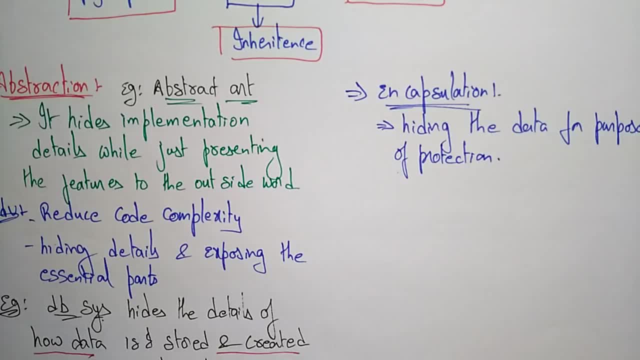 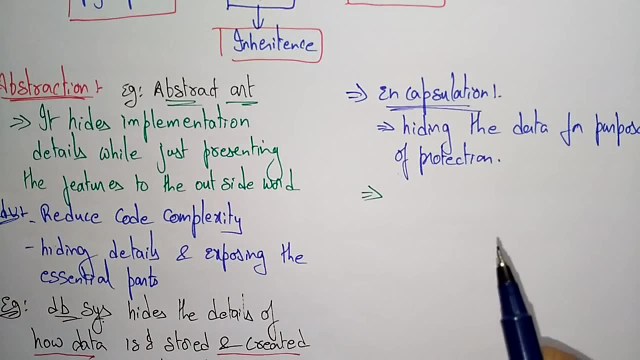 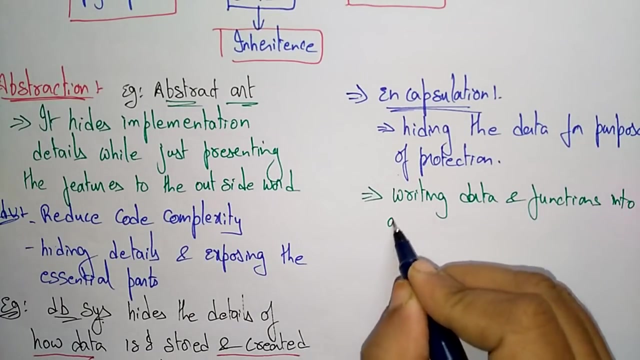 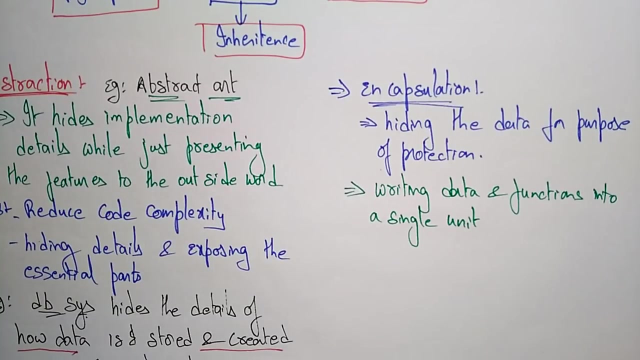 purpose of product or protection. the main concept of encapsulation is here. encapsulation will binds the data. okay, so here what I can say: writing data and functions into a single unit. so whatever you want to write that, the data and functions. so suppose, if you take a structured programming or a procedural 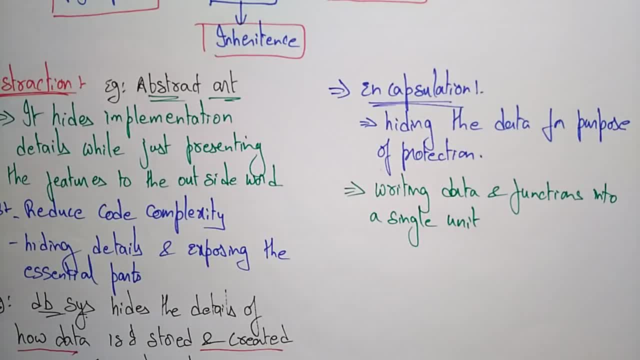 language program. so the statements will be in the form of sequence. they are the structured sequence sequence, whereas in encapsulation here, whatever the data that the program we are using- okay for reusability and maintenance- all the data and functions will be maintained in a single unit. 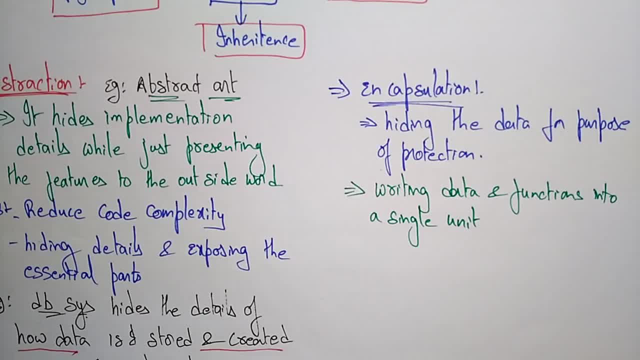 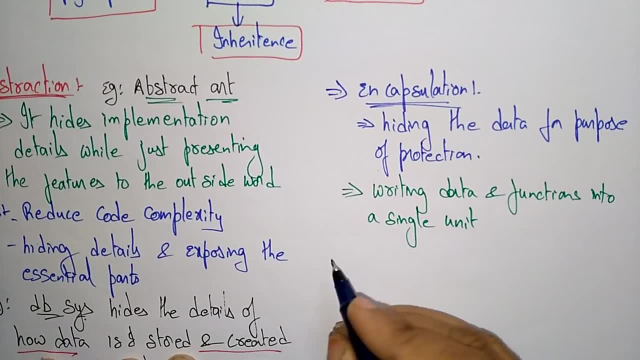 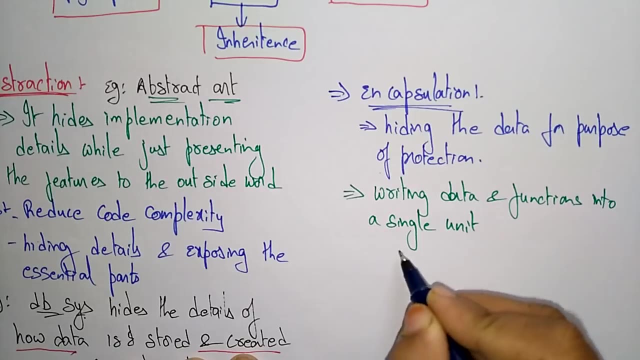 that you call it as an abstract, sorry, encapsulation. so here you can take the simple program like it is. a encapsulation means so let us see the program like it is a encapsulation means so let us see the program here: encapsulation is nothing, but it is writing data. so writing data means data is nothing but it. 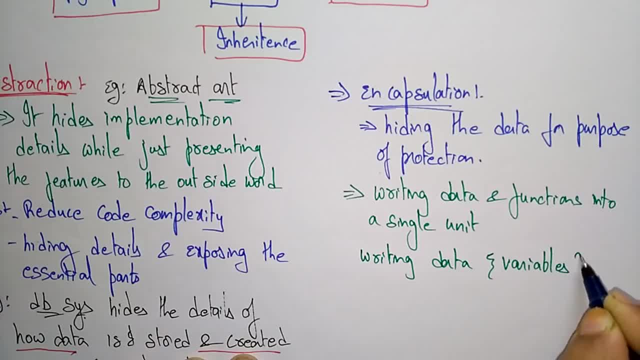 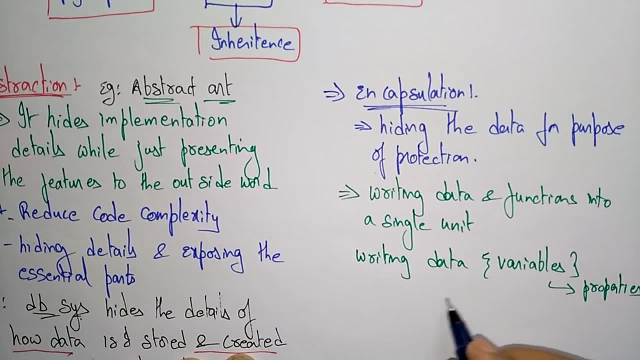 is a variables, variables, variables or nothing, but is having set of properties, like some different variables that are created. so writing data plus functionality. functionality means that you call it as methods. these are all bind in a single unit. that call as a class. okay, these are all bind in a single unit. okay, in the in represented as a class. 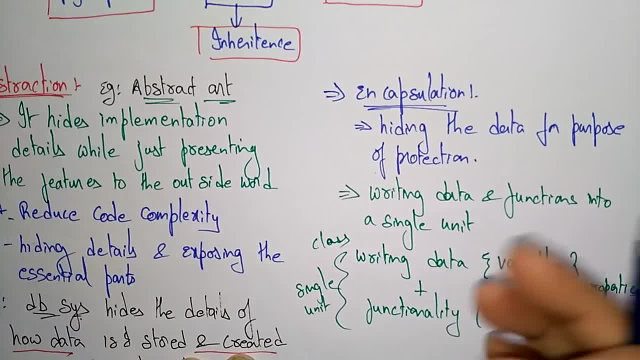 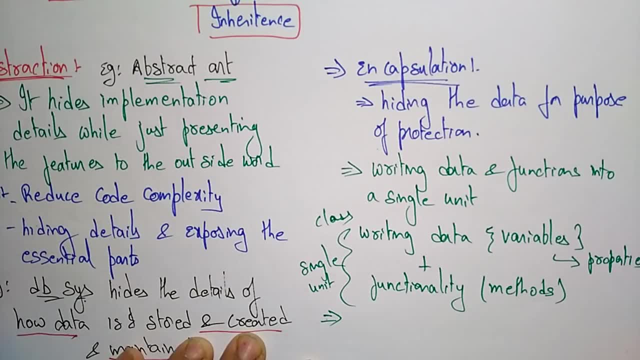 okay this, you call it as encapsulation. so what is the difference between this class and encapsulation, difference between the class and encapsulation? so class is nothing, but class is nothing but model of objects. class is nothing, but it is a model of object. so then, what is encapsulation? 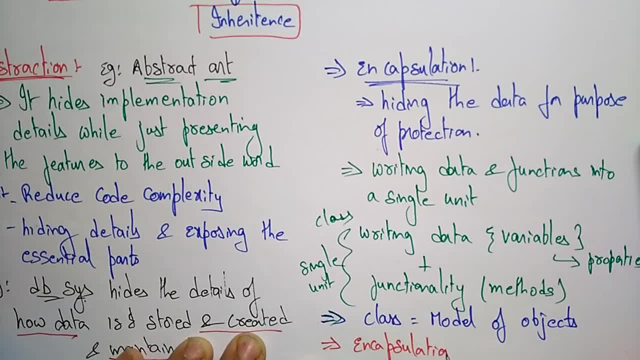 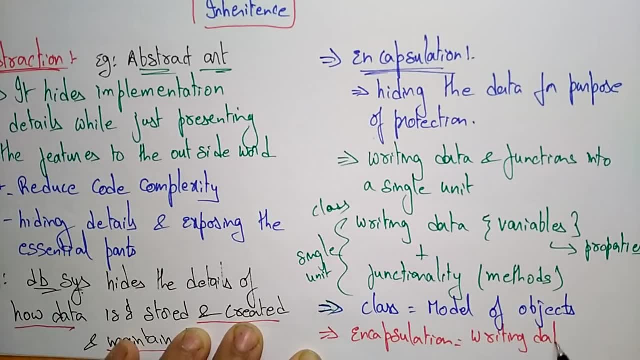 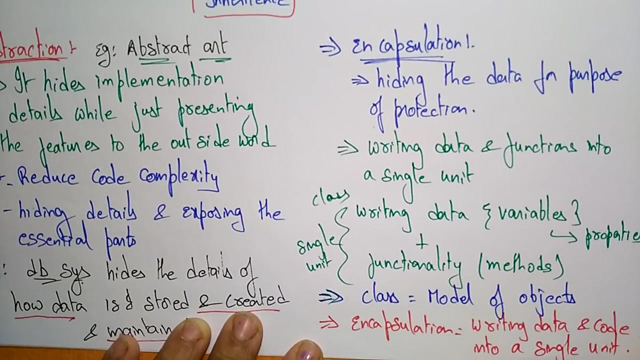 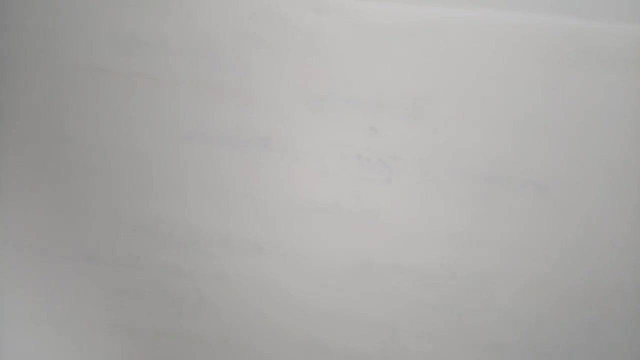 encapsulation is nothing but writing data and code into a set of variables, a set of variables, single unit. okay, so class is a model of object, whereas encapsulation is writing data and code into a single unit. so actually the implementation wise, if you take, uh, in the form of implementation wise. 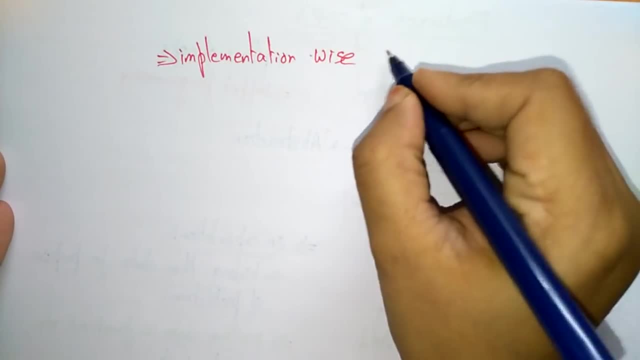 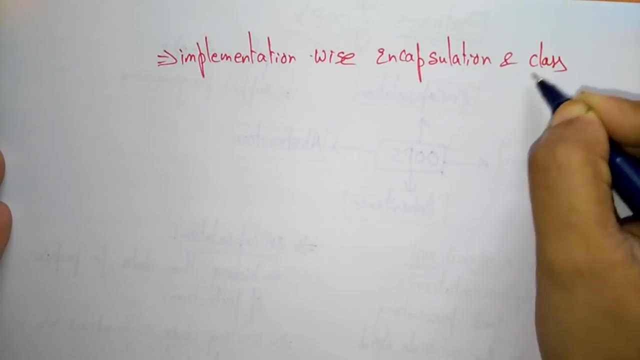 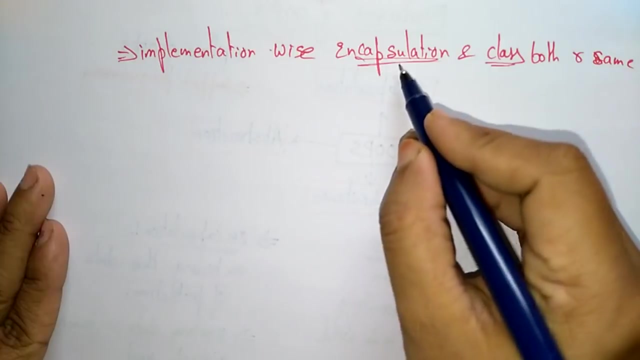 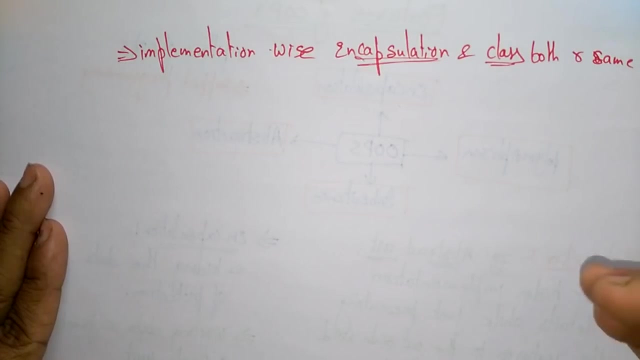 implementation wise, encapsulating and class, both are same. okay, if you think, if you see in the form, in the way of implementation wise, both the encapsulation and both are the same. it's also the hiding, the details, like the variables and the functions, whereas class is also hiding the details of variables and the. 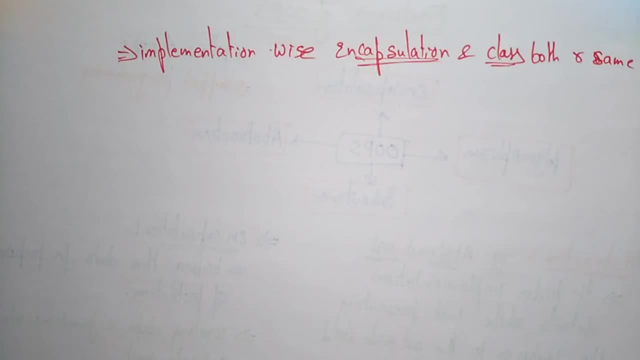 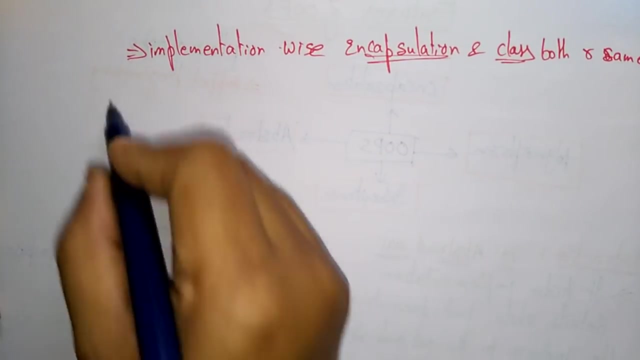 functions means not hiding, it's just placing the variables and the functions into a single unit. the encapsulation and the class is we are writing the data and functions into a single unit. okay, so let us take one example to explain for this encapsulation. suppose if you are driving, 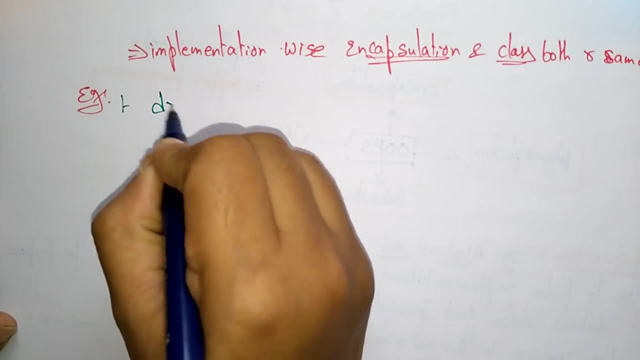 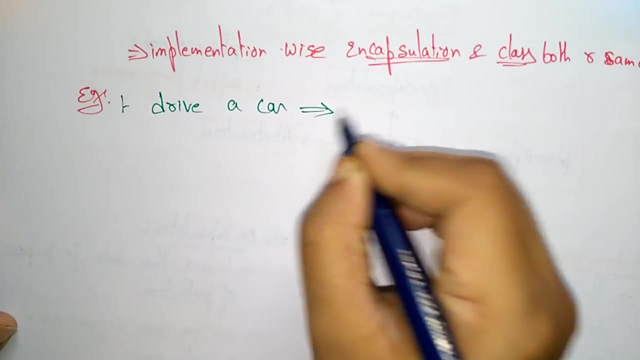 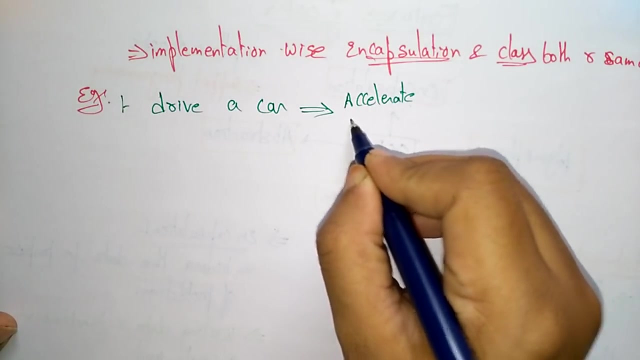 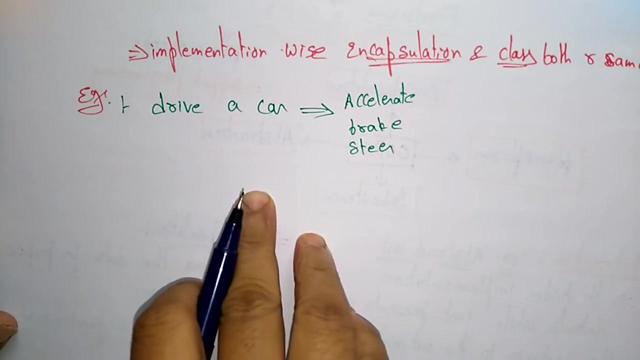 a driver is drive a car, if you take example as: drive a car, okay, so what's the car is having? this car is having to drive a car. we need the accelerator. accelerator and brake and steer steering. okay, to drive a car. a car is having a car, have accelerator.